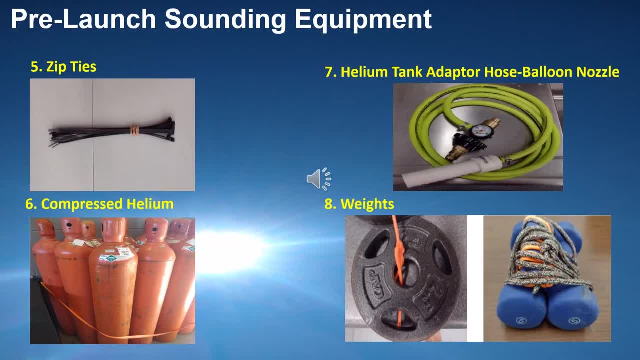 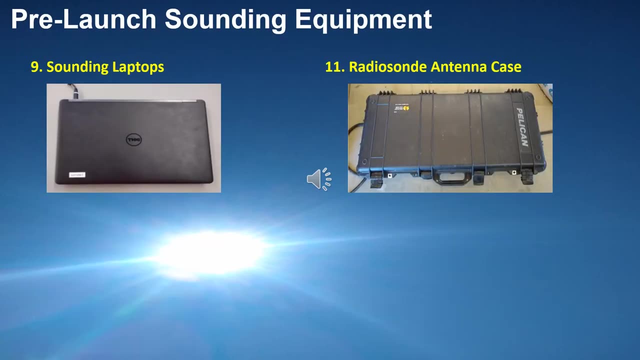 Furthermore, you'll need zip ties, adequate compressed helium, a helium tank adaptor hook and a heat sink. You'll also need the following equipment: You'll need a balloon nozzle and the weights as pictured And finally, we need the sounding laptops, the clippers and a radiosonde antenna case. 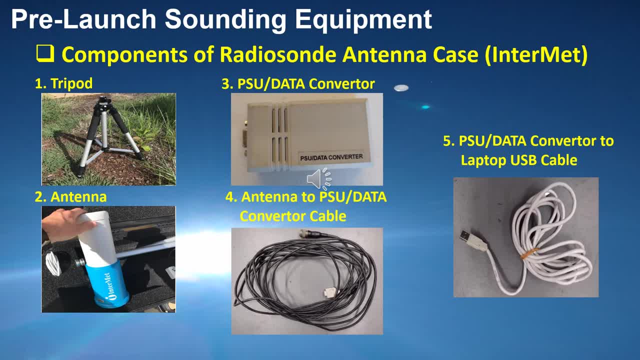 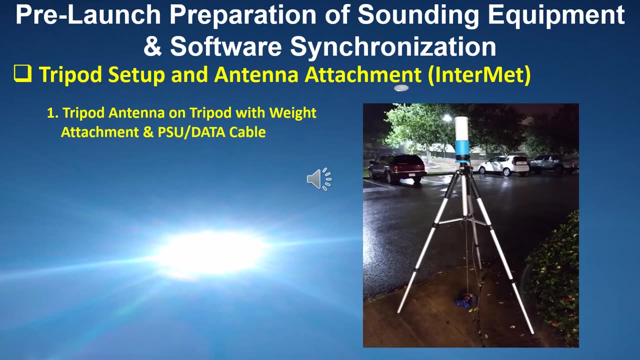 Components of the radiosonde antenna case include the tripod, the antenna, the PSU data converter antenna to PSU data converter cable and the PSU data converter to laptop USB cable. Here is an example of the antenna mounted on the tripod being secured to the ground with a weights system and the PSU data cable connected. 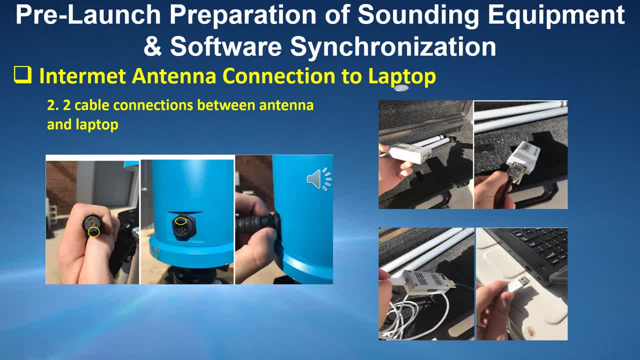 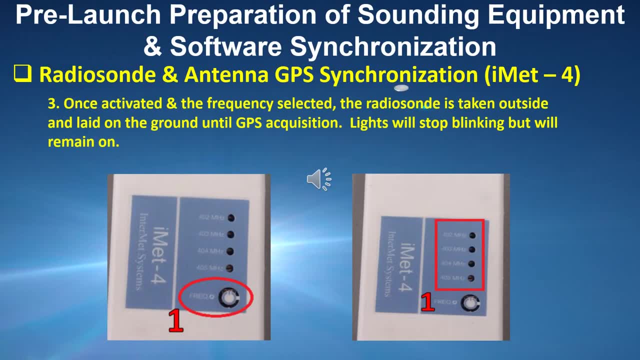 Here are some of the images of the cable connections between the antenna element, PSU data converter and the laptop. Once activated and the frequency selected, the radiosonde will be taken outside and laid on the ground until GPS acquisition. Lights will stop blinking, but will remain on at this point. 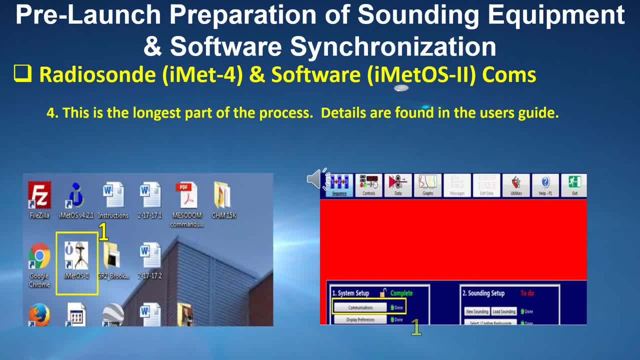 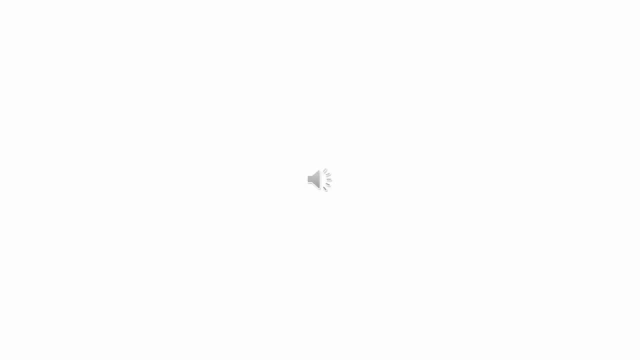 Establishing the communications links between the radiosonde and the software is the longest part of the process, but many of the details are still to be discovered. This is part of the process, but many of the details, or all the details, are found in the user's guide. 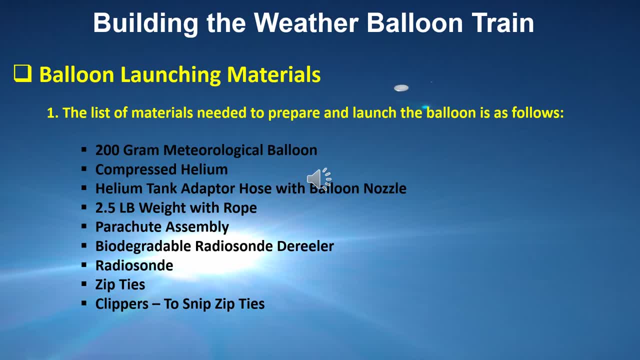 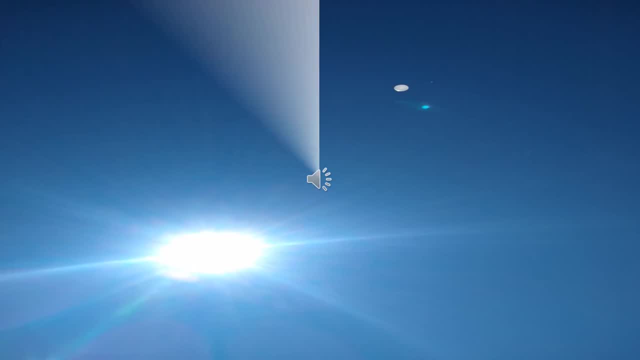 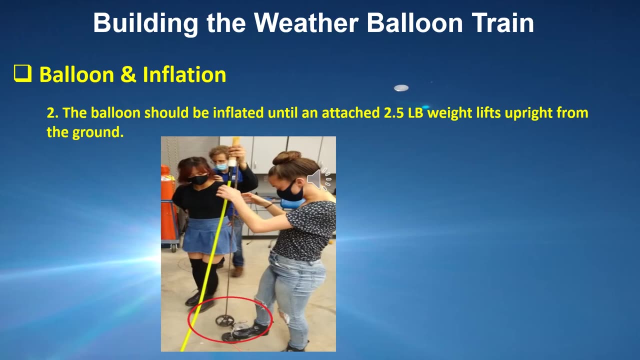 We are now at the part of the process where the previously gathered up balloon launching materials are going to be utilized to create our balloon train. The 200 gram meteorological balloon will be inflated with helium until the attached 2.5 pounds of helium is released from the balloon. 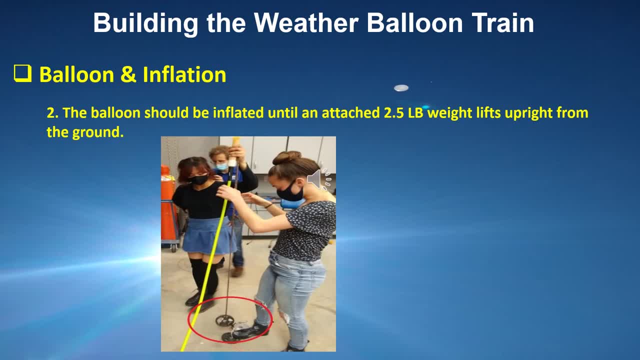 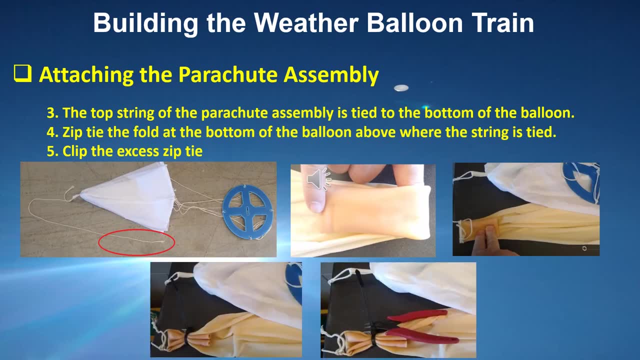 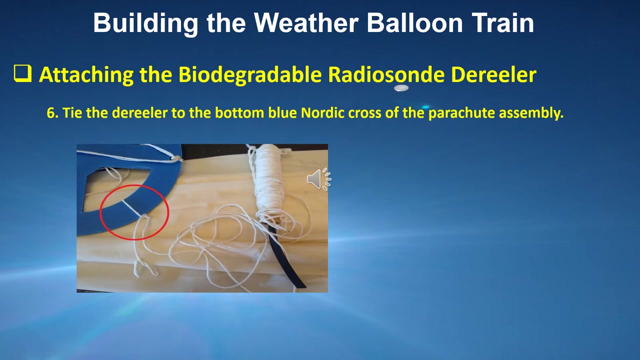 weight lifts upright from the floor. From top left to bottom right are images and how to attach the parachute assembly to the balloon. More details are found in the user manual. The string at the end of the derailleur is looped around the blue iron cross of.